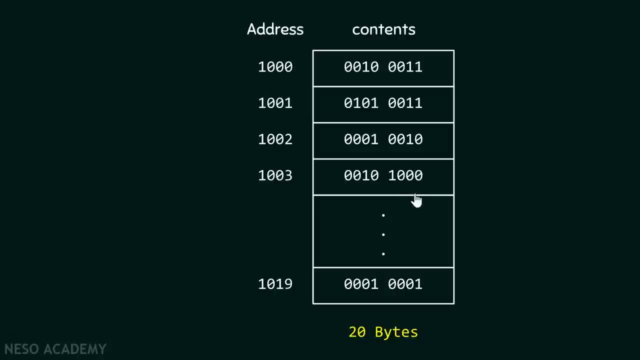 integer will maximum to maximum take two bytes of memory, That is, it will take two blocks of memory For storing an integer. I am taking one variable, i, which is of integer type. Therefore it is capable to store an integer And I am assuming that it will take. 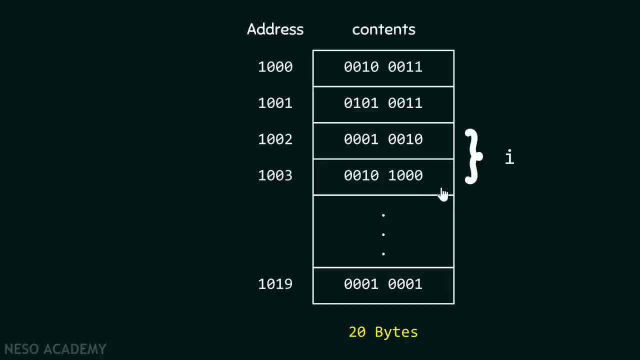 these two blocks. Now let me tell you what a pointer is all about. Pointer is a variable which is capable of storing the initial address of the object which it wants to point to. In this example, I am assuming that I have a pointer which will point. 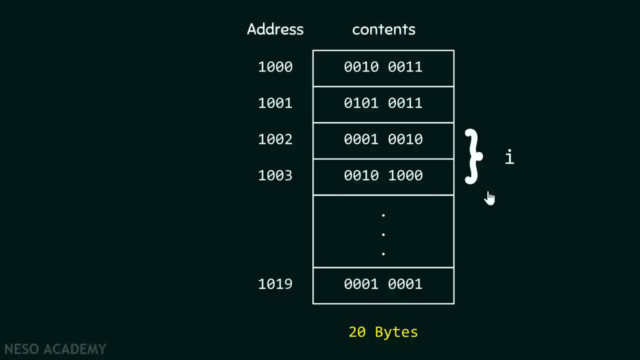 to this particular object, i, And for this purpose, it will simply point to the base address or the initial address of this object, which is one thousand two. Pointing to means it will simply store the base address or the initial address of the object. 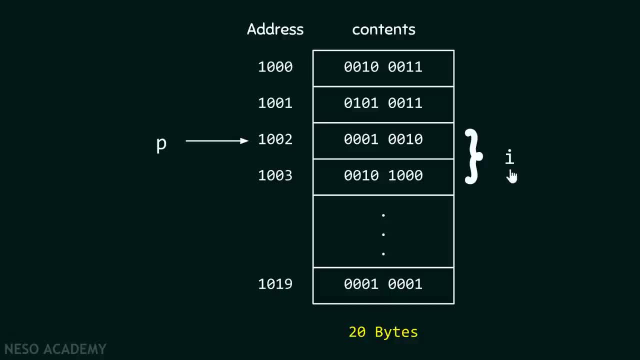 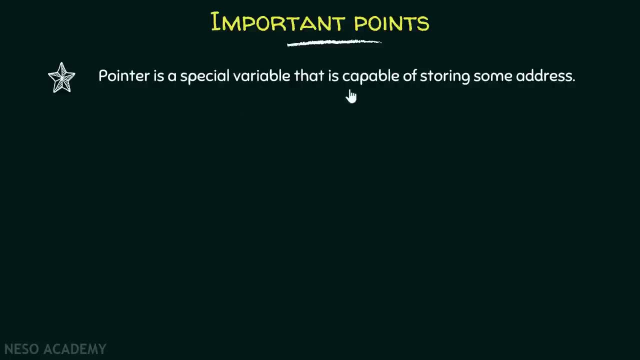 In this case it is variable i. Now let me give you the definition of a pointer. Pointer is a special variable that is capable of storing some address. In our example, it is storing the base address of integer variable i. It can store the initial address. 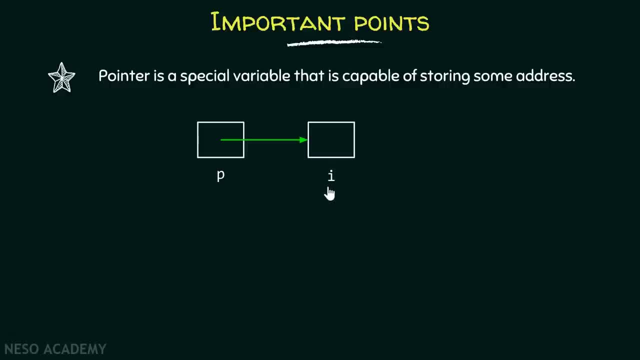 of any object. But in our example it is storing the initial address or base address of integer variable i. It is a special variable. It is not a normal variable which will store integer character or a float. It will store the address or the base address of the variable. 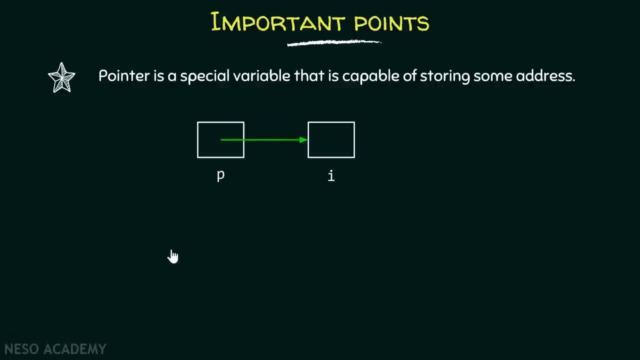 or an object which it wants to point to. Also, it points to a memory location where the first byte is stored. That is, it simply points to the base address of the variable. In our example it is one thousand two. In this lecture I just want to give you. 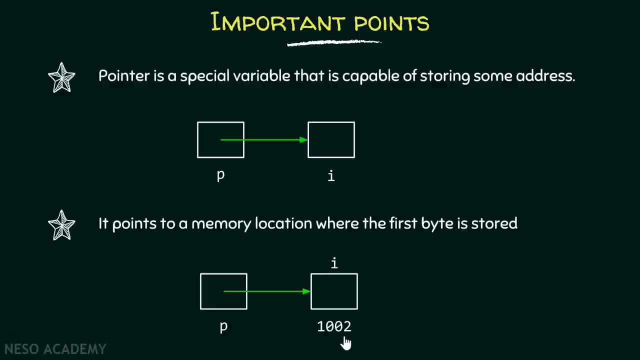 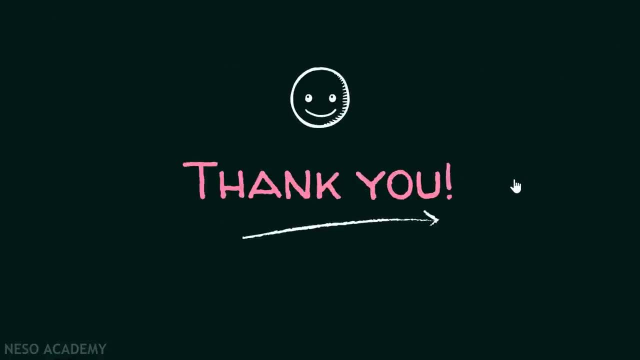 the glimpse of what a pointer is all about and how to imagine a pointer. In the next lecture, we will start with how to declare pointers. Okay, friends, this is it for now. Thank you for watching this presentation.